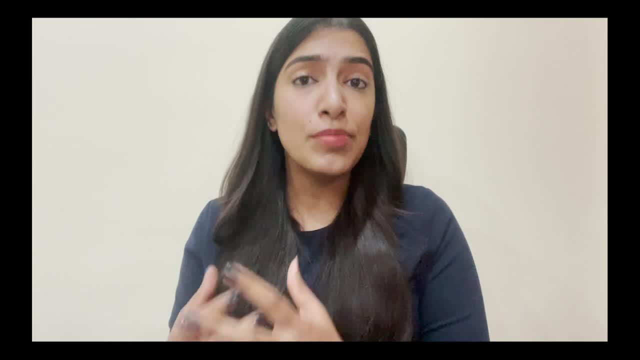 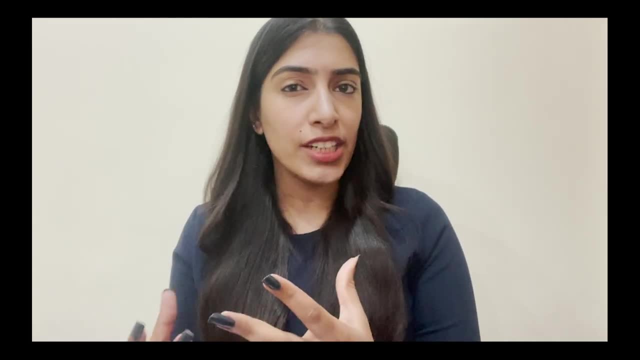 a lot of implementations. for example, there is a db connection. now you want only one db connection to be used by all the modules of your project. or, for example, there's a configuration manager. there should be only one configuration manager which can change the configurations, otherwise you'll. 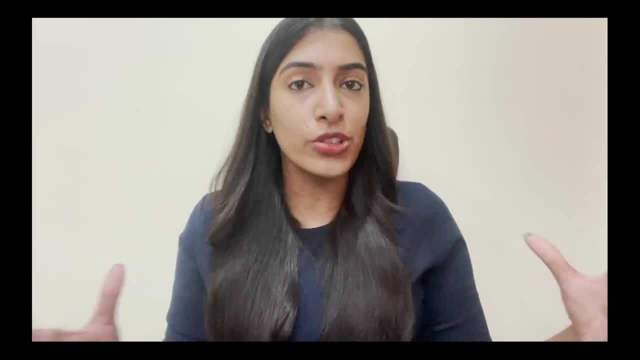 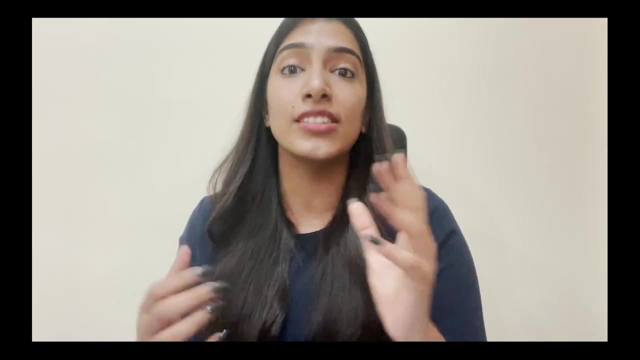 end up having a lot of problems, right? so the entire project, all the modules, should have only one configuration manager. or you do a lot of logging in all the systems, right? so there should be only one logger that is used so that all the logs go in one particular place. 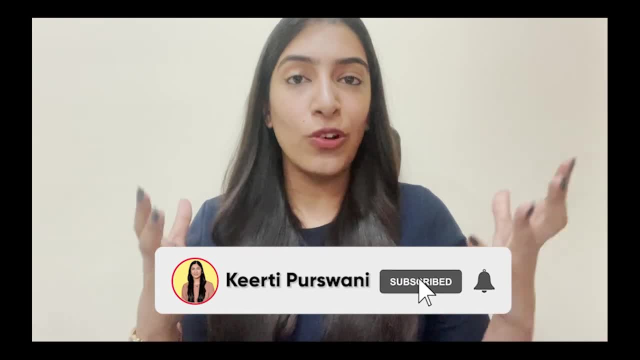 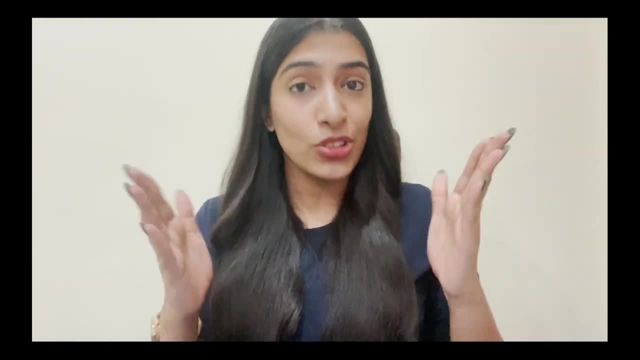 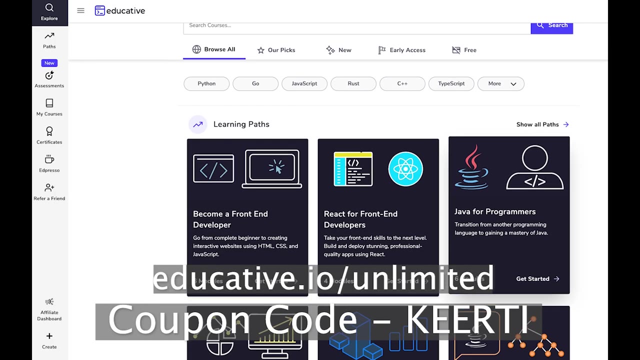 right. so in our case we'll be taking the classic example of logger. we'll be implementing logger using singleton design pattern and we'll go through all the details of the implementation using code. but before that, let me tell you about the sponsor of the video. educativeio has a lot of cool courses for software engineers. i specifically really 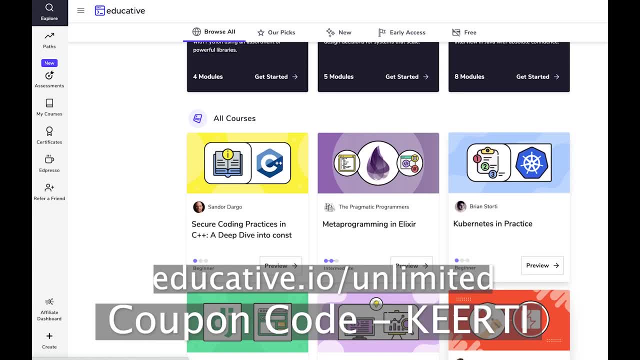 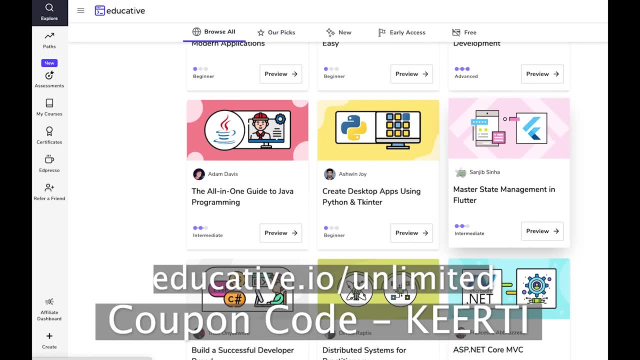 really like their lld and hld courses. that is the system design course. don't forget to use the coupon code kirti to get discount on subscription and get access to all the courses on educativeio. use the link in the description and i really hope it is very. 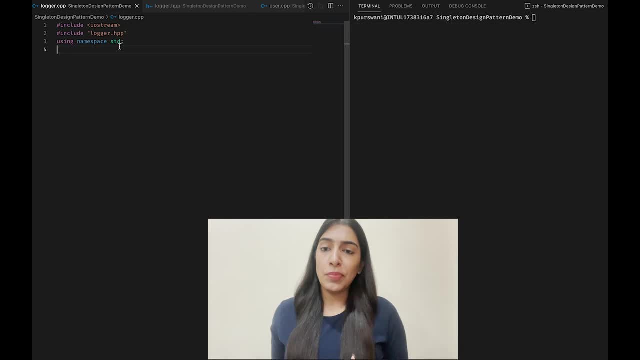 helpful to you. as you can see, i've made three files: loggercpp, loggerhpp and usercpp. let's start with very basic, simple stuff. let's just make a class logger and our user is going to use the class. that's it, very simple stuff. okay, let's start with making the class logger. 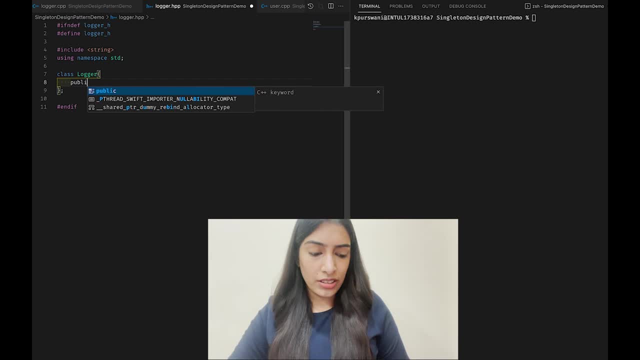 and right now i'm just going to write a constructor in public section. so a constructor, and i'm going to write a log function. okay, a simple log function. you pass a message and it's going to just output that. okay, so void, and i'm going to call it log and i'm going to pass a. 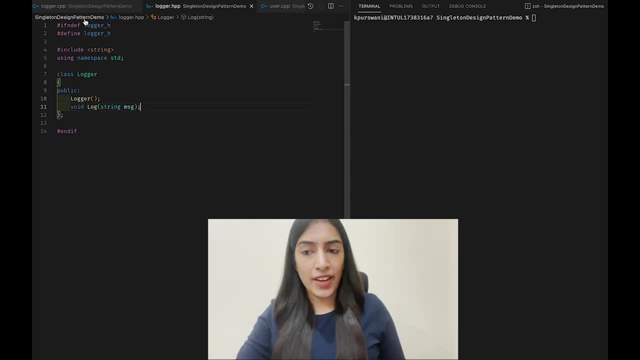 string message to it. that's it. so i've declared it in hpp. let's define it in cpp as well. okay, so let's just start with log constructor and i'm just going to write log constructor and i'm going to output over here that new instance of logger created. so just new instance created, that's it. 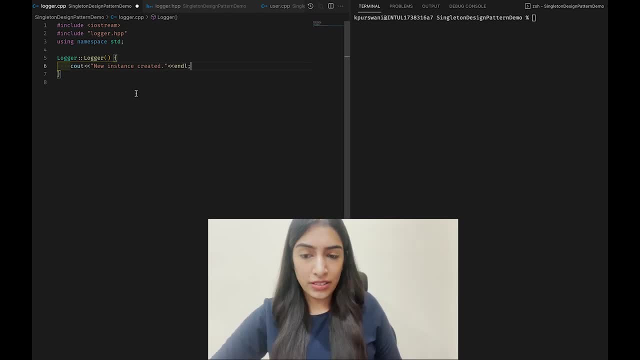 okay, and so it's going to be written. type: void logger and i'm just going to log the message, right? so i'm going to just write output over here: message. that's it okay. so we have made the class and now our user is going to use the logger. 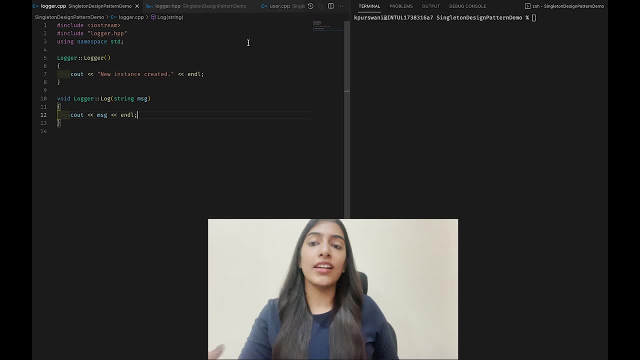 usually there are going to be so many users who are going to use the logger right right now. for simplicity purposes, let's say there are two users and we're going to write the code in the main itself, just for simplicity and for understanding. okay, so what i'm going to do? i'm going to write: 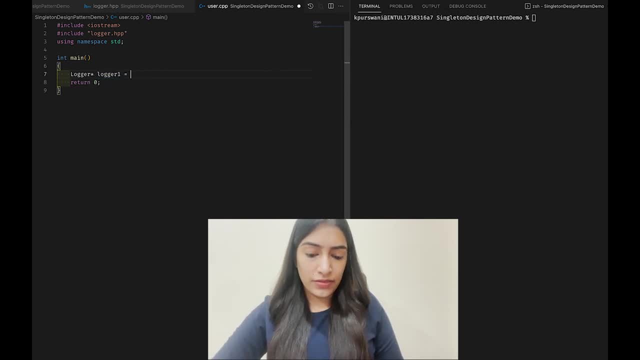 logger1 and i am going to log something from there, right? so i am going to use logger1 to log a message saying this is: this message is from user1 and that's it. okay, i'm going to do same for logger2. so what i'm going to. 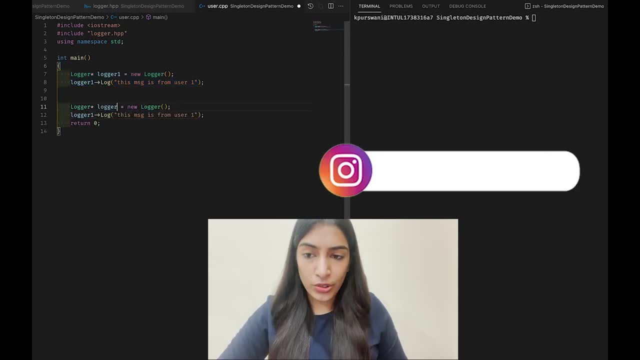 do now is create another logger, which is logger2, and this new log statement is from logger2, that this message is from user2, right? simple stuff, nothing big. i've just made two loggers and that's it, right. so let's compile this and see what happens. 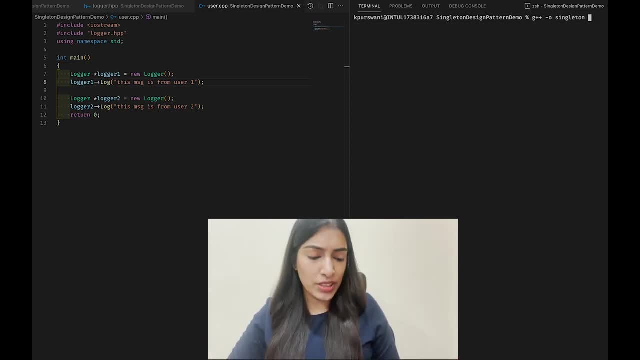 so i'm going to call the executable as singleton itself. just the name of the executable, that's it. and let's run the executable so you can see the output. the two times new instance was created and the messages were from user1 and from user2. right, simple stuff. now see, the entire concept of singleton revolves around. 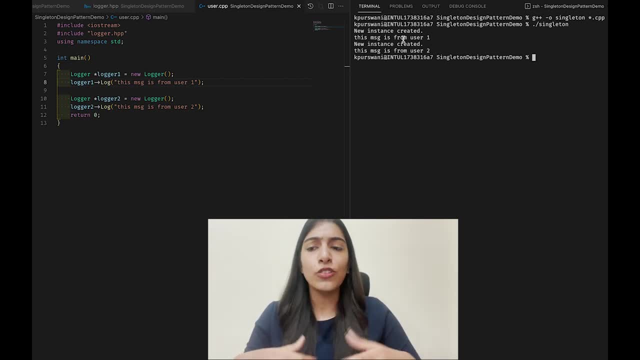 there should be only one instance, right? so there should also be a way to make sure that, okay, only one instance is created. so let's say, for example, someone asks you that how many instances of a class is created, so how do you keep track of that? so for that, what we do is we create a static counter in a particular class. 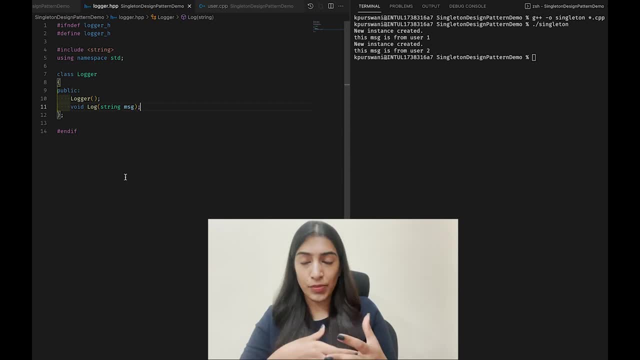 every time a new object is created, that is, every time a constructor is called, this counter value is incremented. to make it very simple for those who don't understand the concept of static, again see: this counter will belong to a particular class and not to an object. so even if you keep 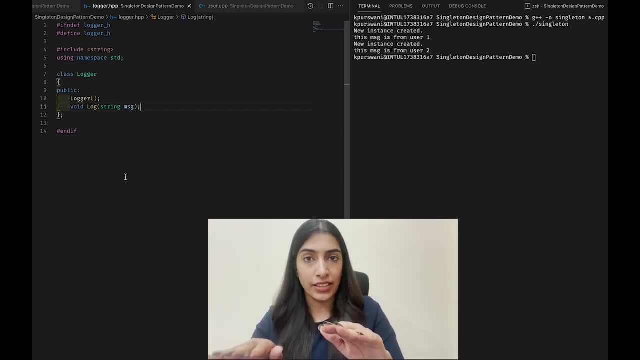 creating new objects of the class. what's going to happen is the counter is not going to get reset. the initial value is just going to get incremented, and i will show it how it works. okay, so if you don't know the concept of static, you're going to learn it now. it's very simple, so i make 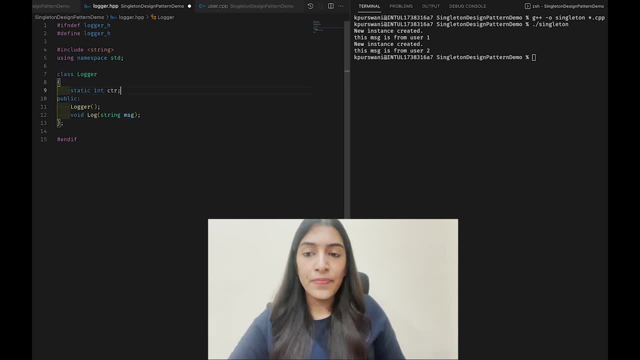 a static integer counter and that's it. okay, and i'm going to use it in cpp. so i'm going to put the initial value as zero and every time the constructor is called, i am just going to increment this value. okay, and i'm going to compute now what the initial value is. now the initial value is zero, okay, so there's. 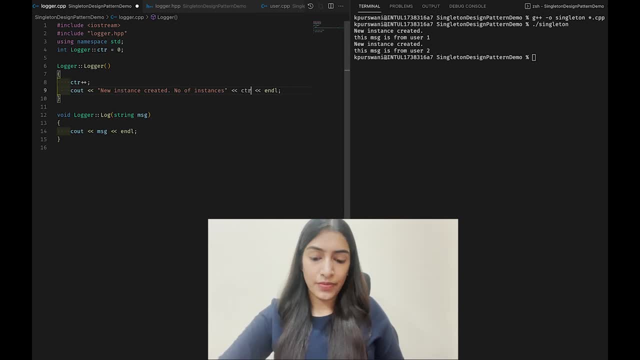 no data, so the number will be put as well. so i'm just going to write number of instances. now is counter value and that's it. okay, now let's see what will happen. so i'm going to compile this and when i run it you can see. now the number of instances is also output, right? so number of? 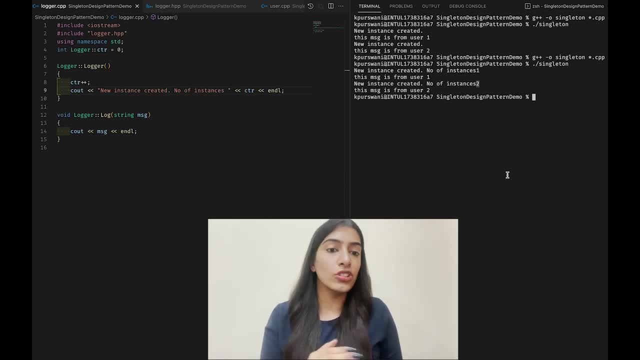 instances. one number of instances is two right, so like this you can keep track of number of instances reset. when the new logger, that is, logger2, was created, the same counter value was incremented because it was there in the constructor. so till now we had a very simple logger class being used. 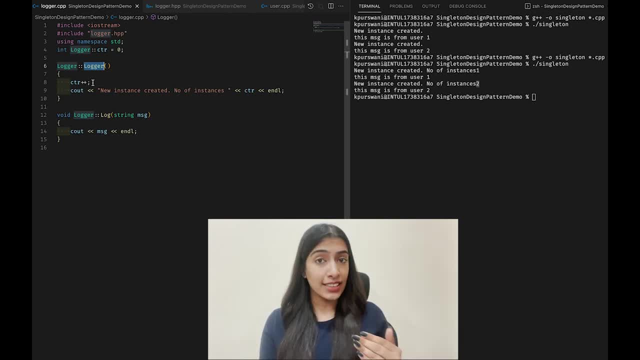 by user. now we are going to make our logger class singleton, so what's the first thing that you can think of for singleton design pattern? first thing is that i don't want my users to be able to create logger objects. okay, i want to restrict them for being able to access this logger constructor. 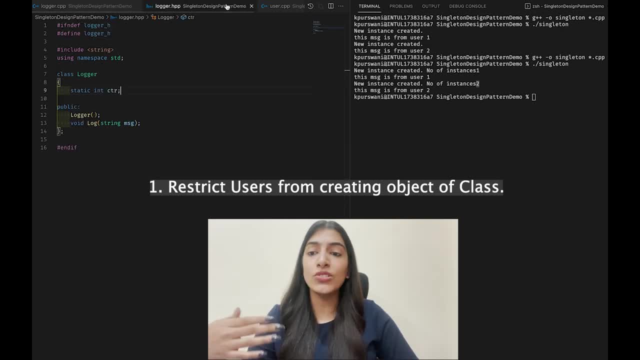 somehow there are ways to do that. one very simple way is to just make this constructor as private. so i'm going to remove it from the public section and i'm going to add it to the private section, and as soon as i save it, you can see the error coming in usercpp. what is the error? the error says that the 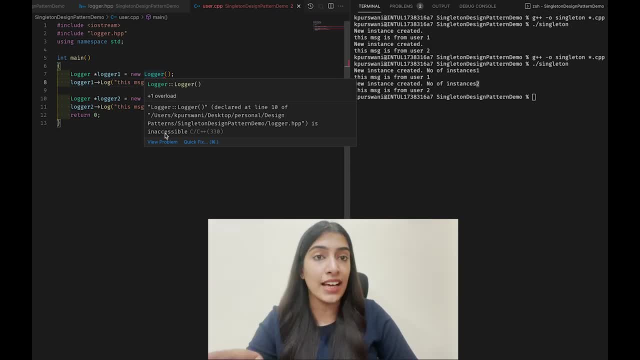 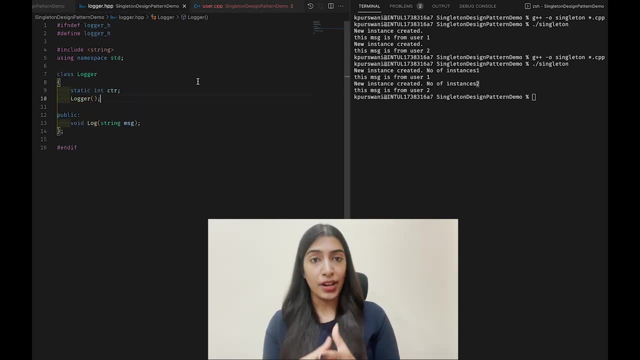 logger is now inaccessible. the constructor is inaccessible. why is that? because now it is private. so this is the first point of singleton design pattern: by making the constructor private, you are restricting the users from creating objects, object, or basically calling the constructor itself. but does that mean that we are not going? 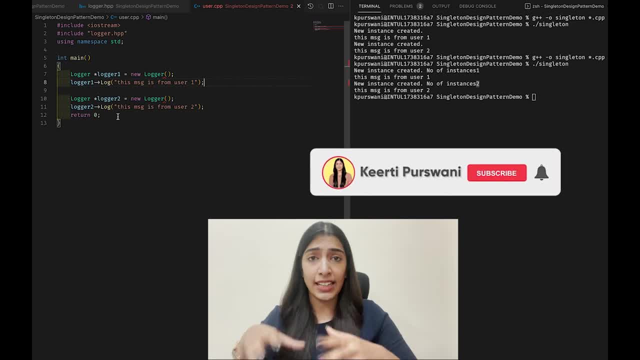 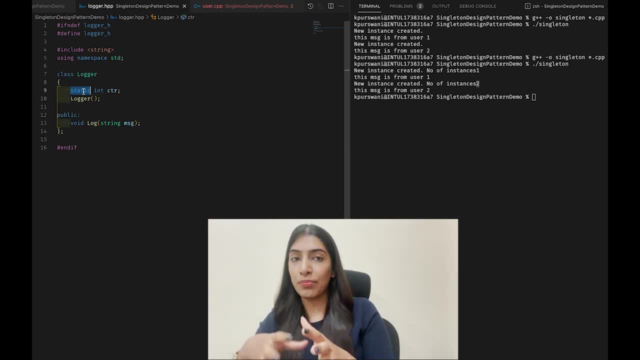 to create logger instances because we do need a single instance right that is going to be used everywhere. so, as i said, see, static property makes sure that a particular member belongs to class and not to a particular object. now we cannot create object because we made the constructor private. 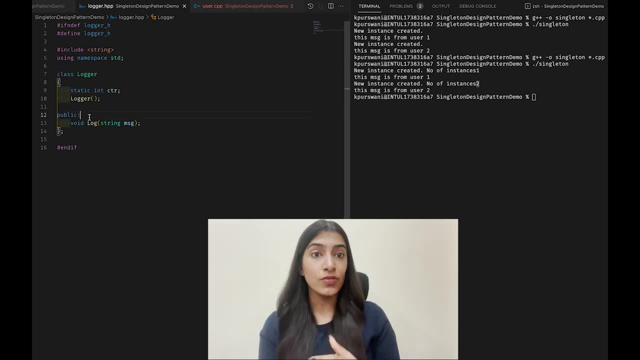 so what we can do is we can make a static function which will return a particular instance, right? if it's confusing, it's fine, just stay with me. it's going to become very simple and easy, i promise okay. so right now i'm just going to write a public function. so i made it static so that it belongs to the class itself. 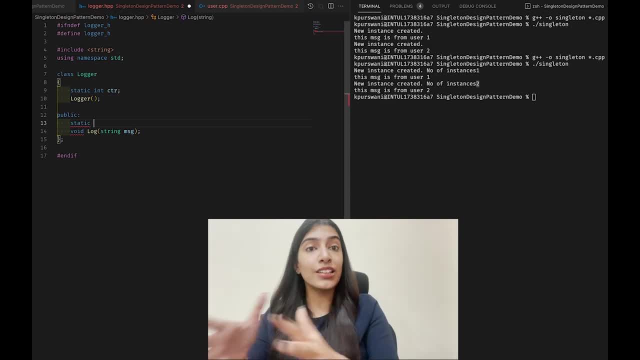 and not to a particular object of the class. okay, so to logger class itself. this function is going to belong. okay, so that's why i made it static what it is going to return. it is going to return a pointer to logger itself. right, it's going to make an instance and give me the pointer to that. 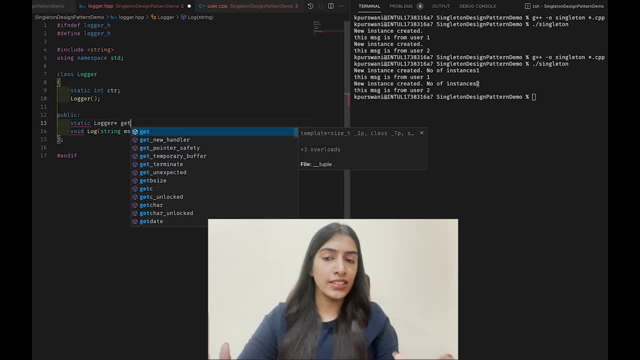 okay now, usually when you see examples of singleton, you will see the function name as get instance, and somehow people start assuming that the function name has to be get instance. so let's keep it different, let's keep it get logger, so that you understand that, okay, it doesn't have to be. 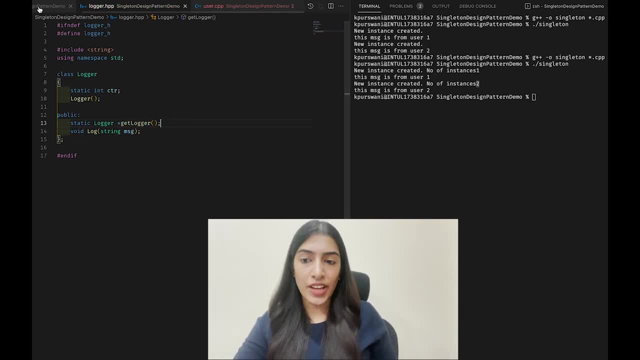 called get instance. okay, so i've declared the function. let's define it also in the cpp itself. so it's going to return a logger pointer and it belongs to logger class and the function name is get logger. right now you need one particular instance to be returned from the static function. 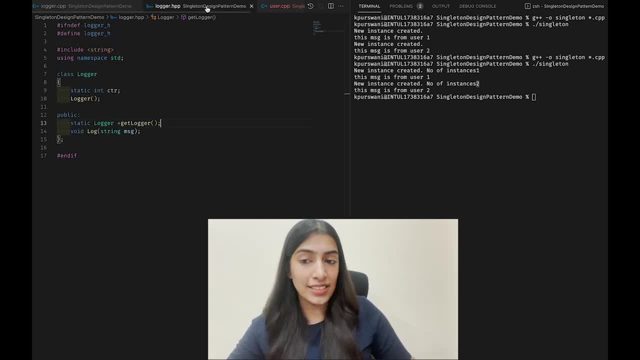 right? so you obviously always also need a static instance itself, right? otherwise, what are you going to return? but that should be private, right? why make it public? so i'm going to make a static instance right now and i'm going to call it logger instance. okay, and this is our single instance that is going 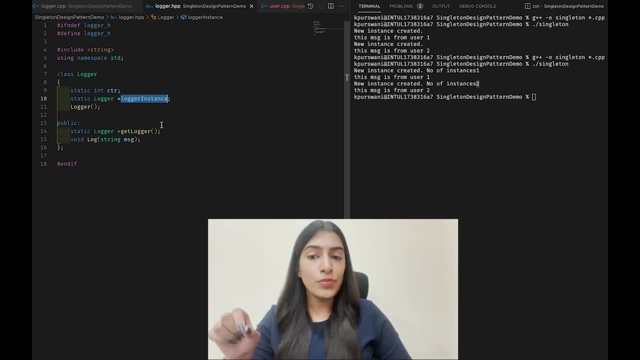 to be used by all the users. okay, we have to make sure that every time this get logger is called, every time we return this one particular logger instance only, there's going to be an instance. okay, we have to make sure no new instances are created, since the instance was. 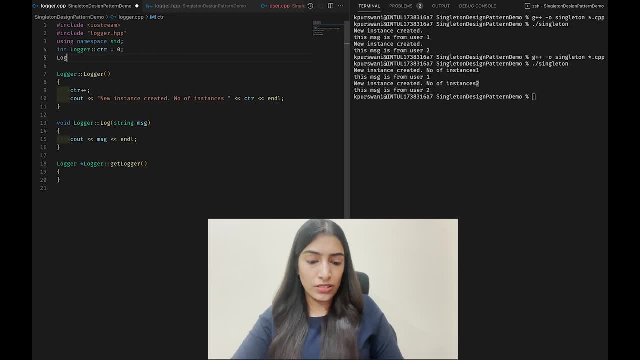 static. let's initialize it in cpp. let's call it logger and belongs to logger and it's logger instance and i'm initializing it to null. okay, now, in this get logger function that is going to be called by all the users, we are going to return the logger instance, okay. 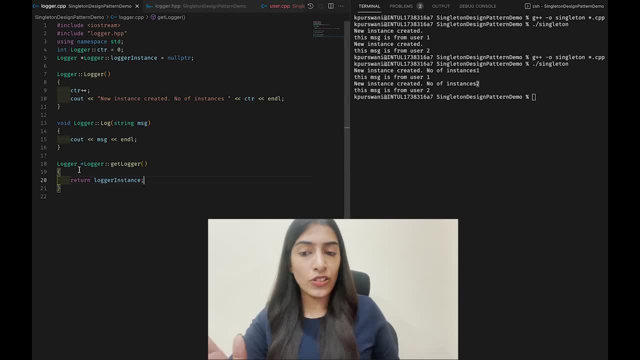 we have till now not created this logger instance. okay, so this get logger itself can do it, but it has to make sure that if it is already created, i just return it as it is. if it is not created, that is, if we are calling the get logger for the first time, okay, so if it is equal to null pdr it. 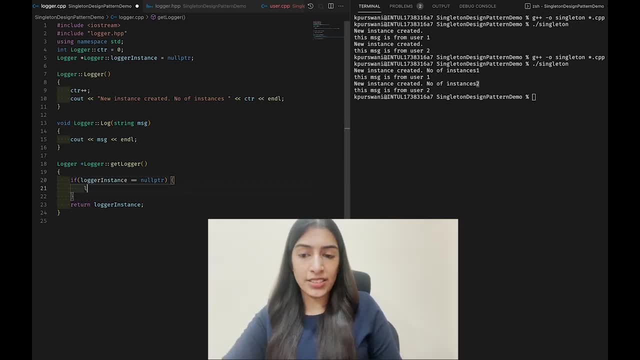 has never been instantiated. what do we do? we instantiate and that's it. see, what happens now is that we check that we have not created the get logger instance. okay, so this get logger instance check that if the instance was already created, we return it as it is. if it was not created, if 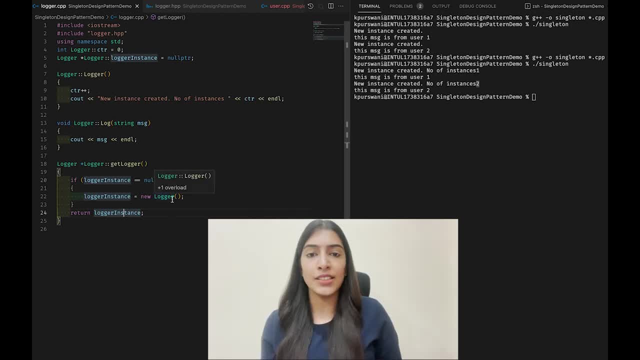 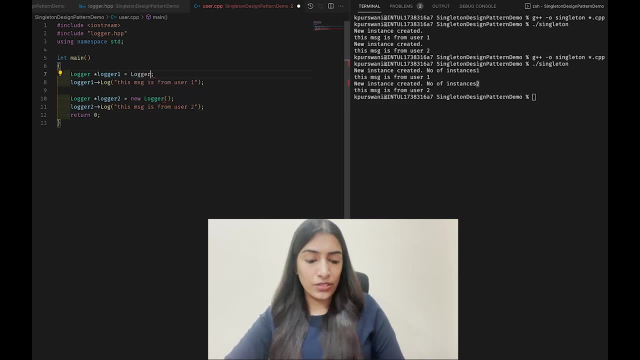 it is equal to null ptr. we create a new instance and we return it. it is as simple as that. and now what our users have to do it: instead of calling new logger, they have to call get logger. see again repeating the same thing. uh, that get logger was called using logger class itself. we did. 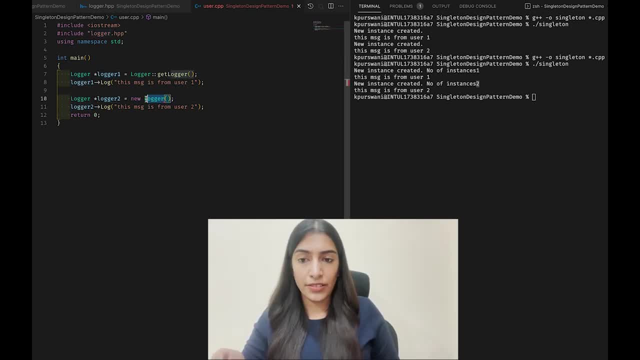 not have to create a logger object. as you can notice, see logger and i do get logger. that's it. okay, let's run now and see what happens there you go. so earlier you could see that there were two instances created, right, so there was number of instances one and number of instances two. right now we have done the. 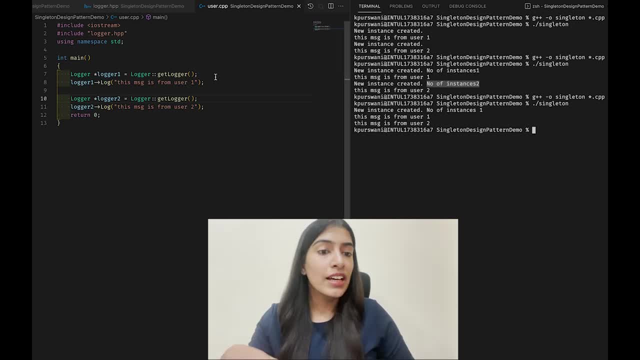 same thing: that instead of new logger, new logger, we have done get logger, and now the number of instances is just one. so now, no matter how many times get logger is called, only one instance, that is, the login instance that we created, will be created and it's going to be used everywhere. 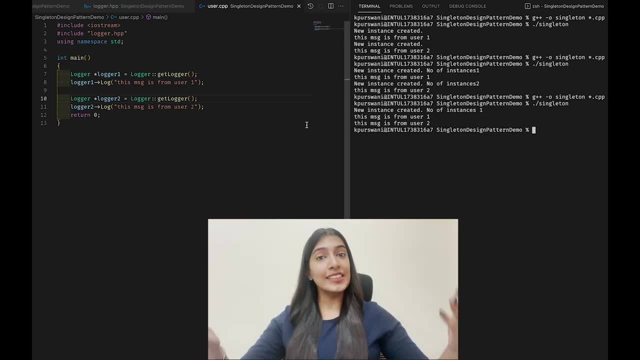 i know that most of you are now very happy that we have already learned singleton design pattern. it was very simple, right. only three steps were there. first, we made the constructor private so that no users can call the constructors. second, we made a static instance and we made sure that only 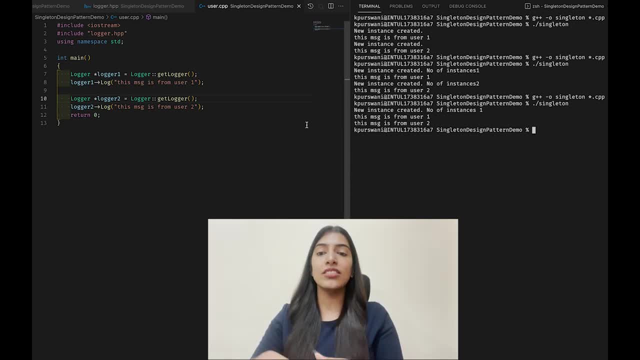 that instance is created by making a static function, which will be now used by all the users, called get logger right. very simple, only three steps, and we have learned singleton design pattern, but is it? no, not really. let's now get to the implementation details. the code that we have written is not thread safe. now i know i'm going to talk about multi-threading. 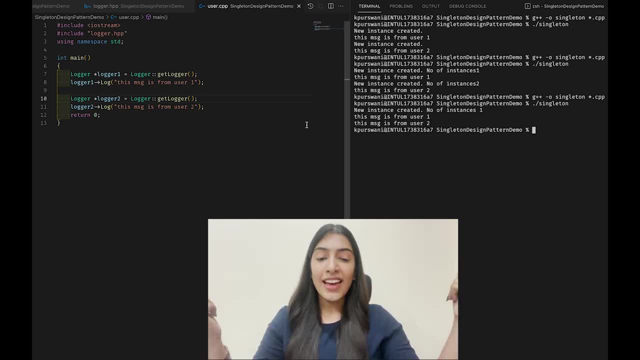 and that scares a lot of people, including me. but i'm going to make it very simple and easy. just stick with me. okay, i'm going to make it very easy. let's see this particular code. okay, the first time we are creating the logger instance. now, suppose there are two threads. 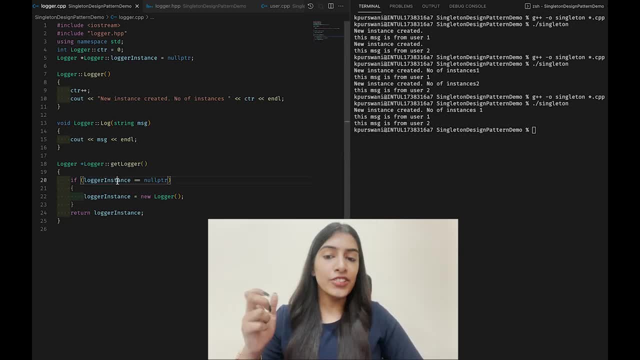 working parallelly and they try to create this instance. the first thread comes and it checks that, okay, this is null, so it starts creating the logger. the second is the second thread comes and now it sees that, okay, till now this logger has not been created, so still, it is nullpedia. so now, second: 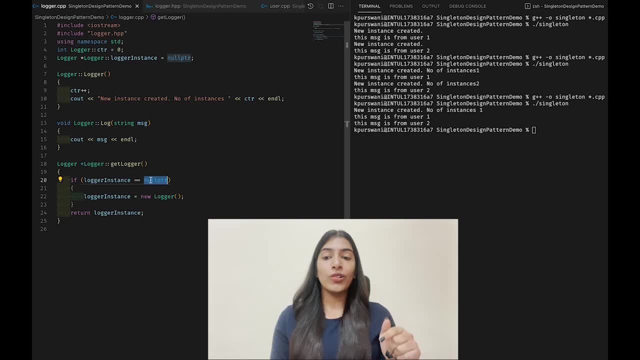 thread also starts creating the instance. so now what will happen is two instances will be created by two threads, which is wrong. we want only one instance to be created by anyone. we want to make instance. so how are we going to do that? this is not thread safe and if you have not understood, 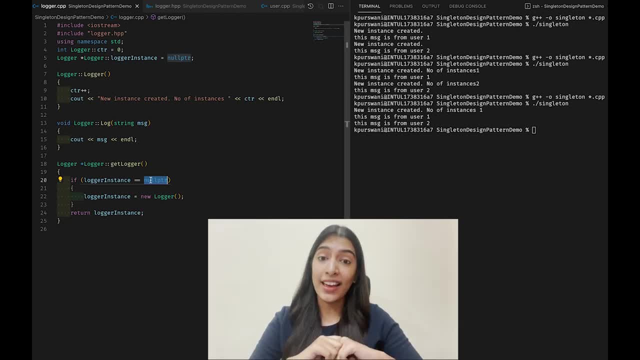 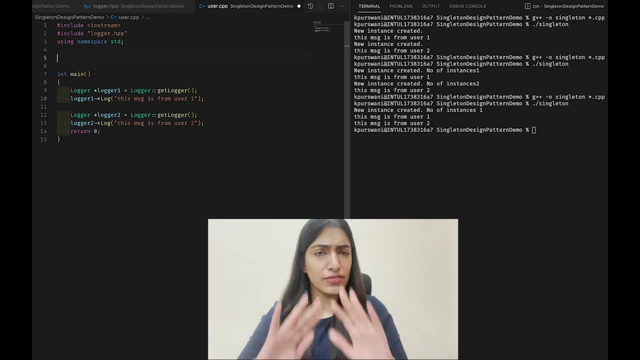 that that's completely fine, because we are going to see it in code as well. now what i'm going to do is i'm going to move these two logs by two different loggers into different functions, just creating two simple functions. don't get confused. so function one is void. 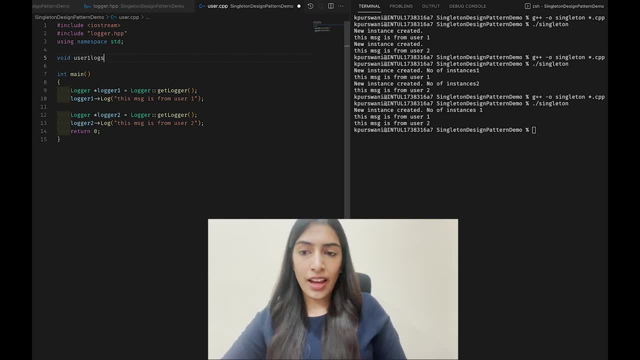 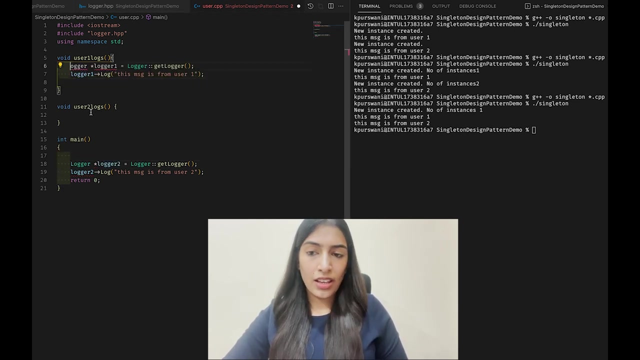 and i'm going to call it user one logs. and similarly, i am going to create another function, user two logs. that's it simple, okay, and i'm going to move this code to the first function- oh sorry, i missed the l- and i'm going to move this code to the second function. 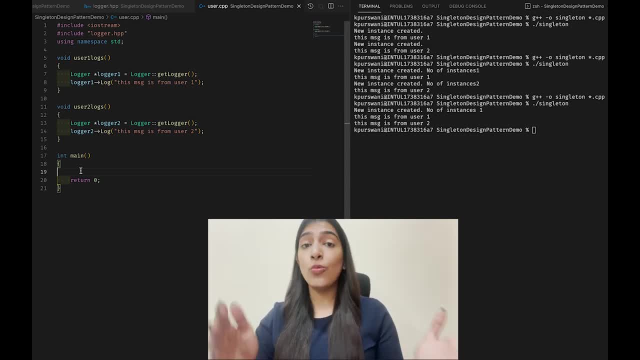 now that we have created two functions. we are going to create two threads now. one thread is going to call one function and the other thread is going to call the other function. okay, let's do that. very simple stuff, don't get overwhelmed on anything. okay, i'm just going to include thread. that's it, very simple. 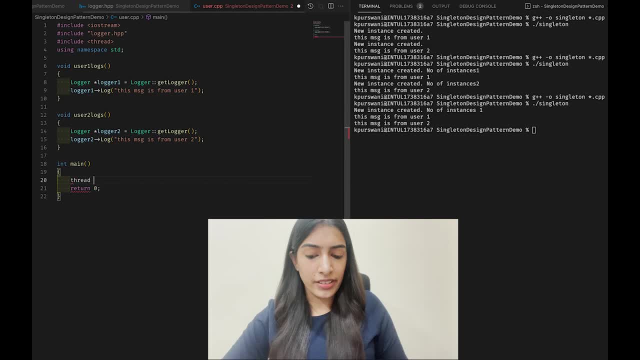 okay and i'm going to create two threads. so i'm going to create thread t1 and i'm going to pass user one logs to this and i'm going to call another thread t2 and i'm going to call user two logs to this. okay, and i'm going to join both the threads. 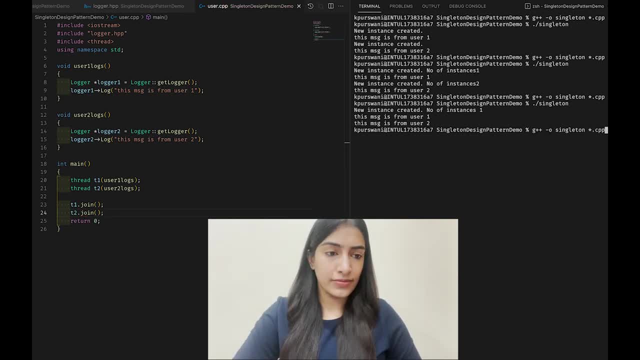 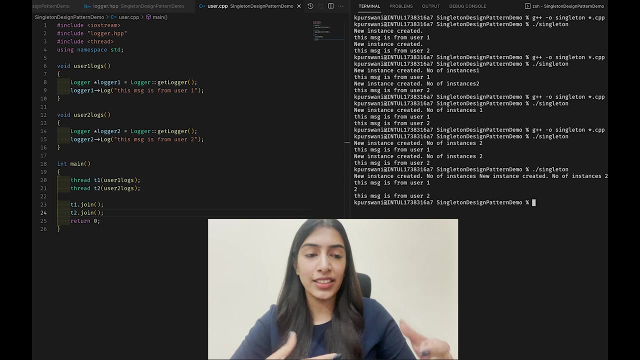 alright. another question i also have when iіл the third part of this, for instance, it's about auditing. okay, see if there is information about the hearth it first and what's going to get executed fast here, if you can see the number of instances got. 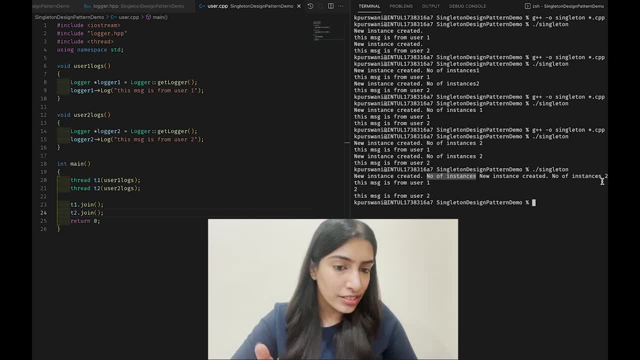 output, and after that the two got output later. this is the two that got output later and here first this thread came and it output this. okay, but anyway, two instances were created, the output was still happening, right, so again, see, now the output is again different. so the number of 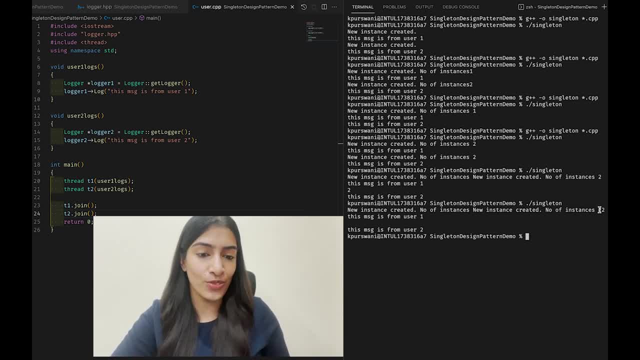 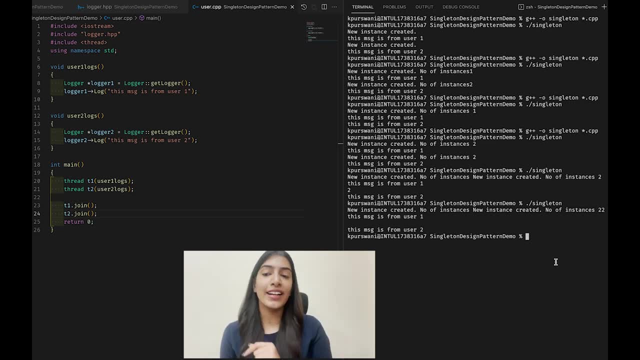 instances two and number of instances two. so that's why there are two twos over here. but interestingly, in all the three times that we tried we actually got the number of instances as two. so you know for sure that our singleton code that we wrote is not working for multi-threading. 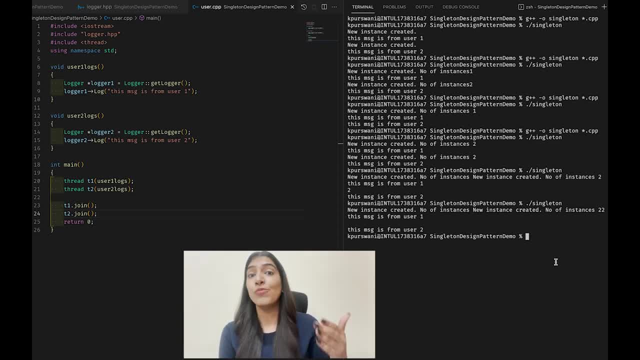 cases, because the number of instances that we created is now more than one. so how do we make sure of that? now, when there are multiple threads, what do we do? we just block a particular code and make sure that when one thread is accessing it, the other thread does not access it. it's as simple as 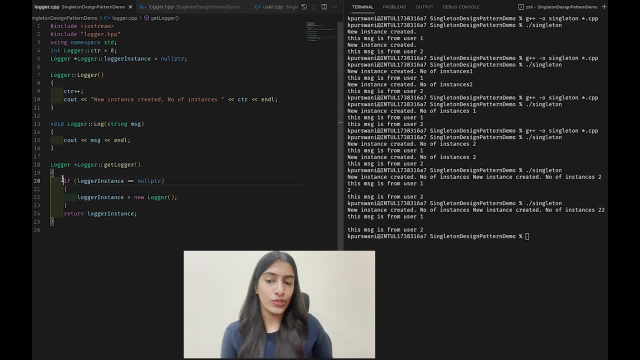 that okay, and in our case, this is that particular code right? you can see that the number of instances that we created is now more than one, and in our case, this is the number of instances that we created. so whenever one particular instance is getting created, we have to make sure that it is locked and no other thread is accessing it. so to put the lock. 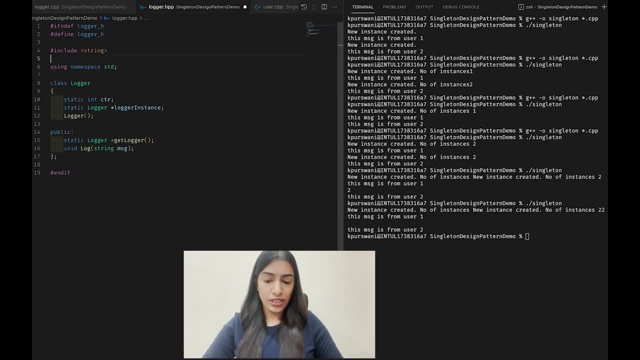 we are going to use mutex, so i'm going to include it over here. okay, and since i have to use it in static function, i'm going to make my mutex as static and in cpp i'll have to define it. so i'm just going to write mutex. 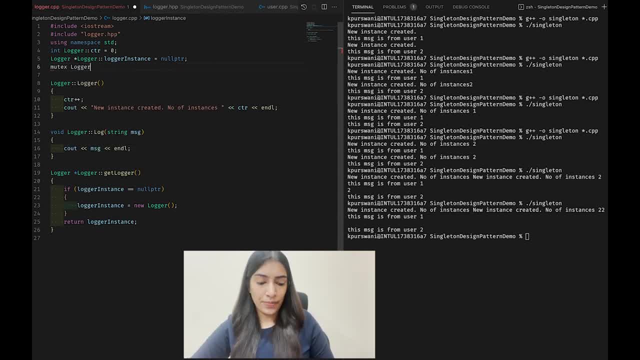 and logo and index. that's it, okay. so i'm going to use this mutex to put a lock before this is getting called and i just unlock it later, and that's it. let's run now after putting lock and see what happens. so i've compiled it now. i run it. see now, number of instances is only one. 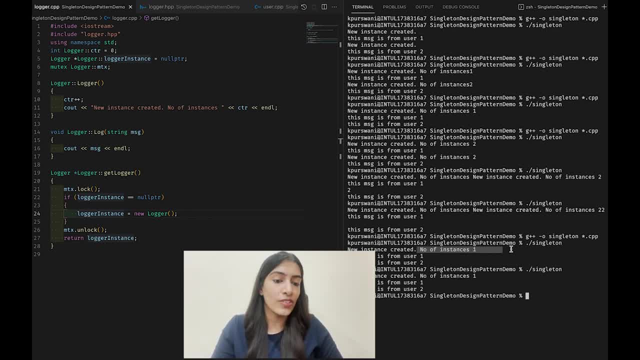 no matter how many times i call it, the number of instances is going to be one. so see, when thread one was trying to create the instance, there was a lock. so when thread two came, there was no confusion and the instance was returned as it is. so second time instance was not created, so we have handled a. 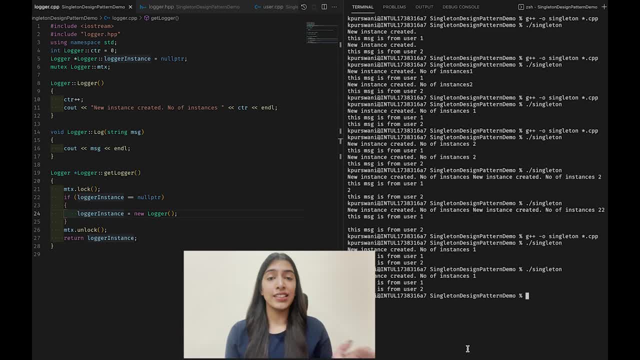 multi-threading situation. see before, we started talking about multi-threading and right now the only difference in the singleton class is about this one particular lock. all we have done is that we have put the instantiation of the logger instance inside a lock and that's it, and we have handled the multi-threading scenario right. i know right now you're very happy. 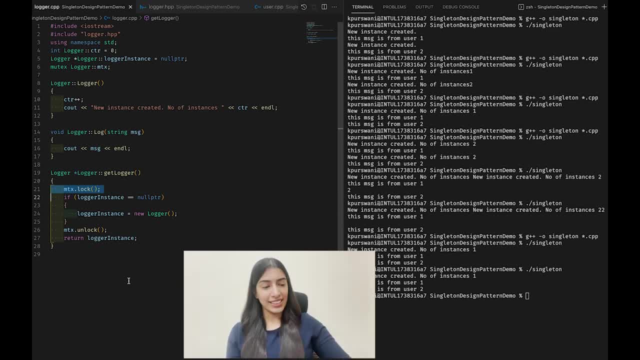 that you have already understood singleton design pattern, but again, this is not it. if you write this code, there is going to be a question that will be asked in your interviews as well as your code reviews: that see now, do you need this lock all the time? because the first time the instance is 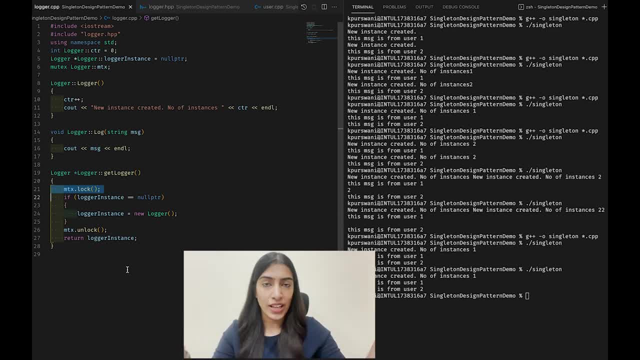 created. there is problem, right that? okay, two, three threads might be trying to access it at the same time, but once the instance is created, you don't need to do anything else. you don't need to do anything. you don't need to put lock at all. you don't need to put lock before the check itself. so now what you? 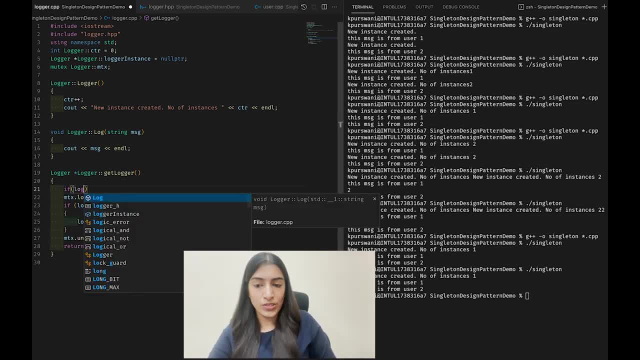 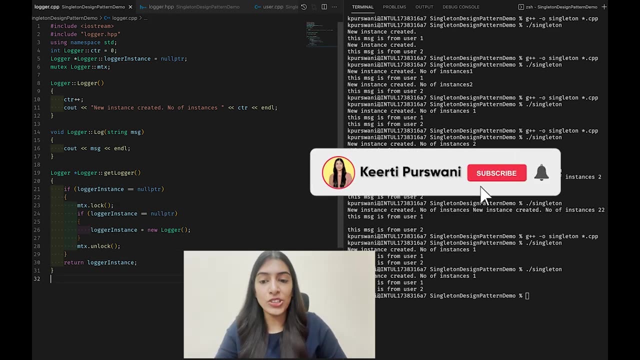 do is you put a check outside as well, so you just check that if logger instance is null, and only then you put the lock and you create this and this, my friend, is called double check locking, because you are checking the logger instance is null or not, two times one is before. 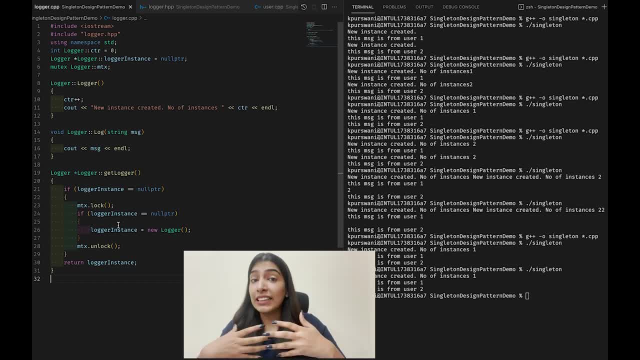 putting the lock. and next is after putting lock. see, because you have done this two times, you have done this two times. do it right there and after doing it it will become horizontal or whatever. so in principle, you have done what you are checking the log, so you cannot. you have done. 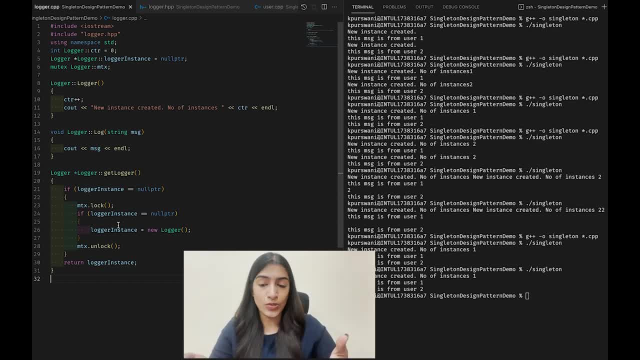 the lock inside, because locks are really expensive. now what you are doing is that you are going to put the lock only once. that is the first time. what did we do till now? we had to make sure that only one instance of logger is created, so we put. a check that if it is null, only then you create the new logger. otherwise you return the logger as it is. then we realize it is not thread safe, so we put a lock outside. then we realize if thread is this kicked, we are going to build the log out as well. this is okay, all right, so we now got the log and down starting to 9 consideration. now in the tool we defined log outside, so we only need to complete a little know one. don't look, start certain, we are going to put one log without adding the log. 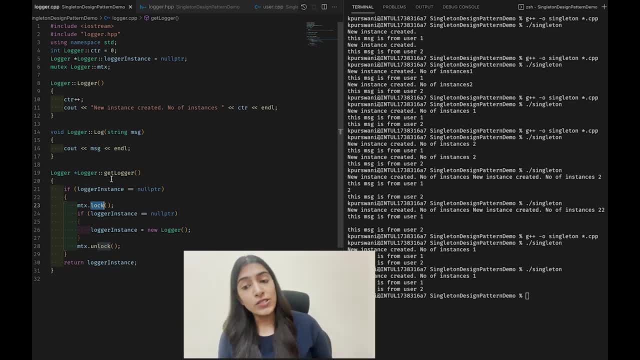 realize that putting locks is really expensive. so we put a check outside also to make sure that we put the lock only the first time and after that we don't put the lock. okay, is it clear now? so we have to check whether it is null or not, and then we put the lock, and then we check again, and then 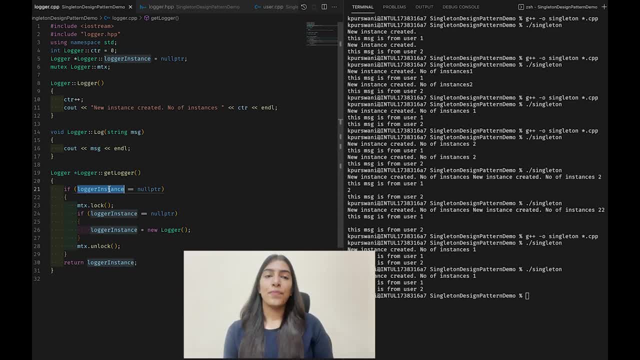 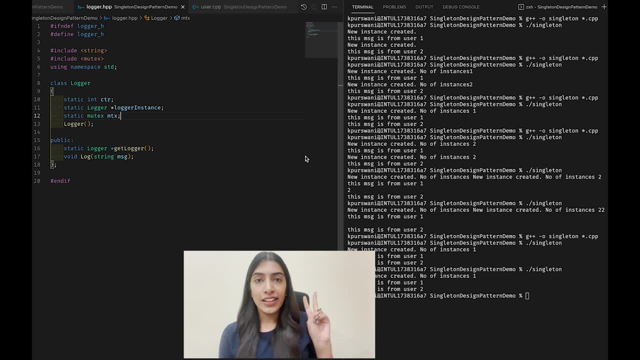 we clear the lock up, that's it, damn almost. you are still not done with handling all the cases. even now there can be problems. there are two more important points. point number one is: let's see this default constructor is not the only way to call constructors right, and we want to restrict. 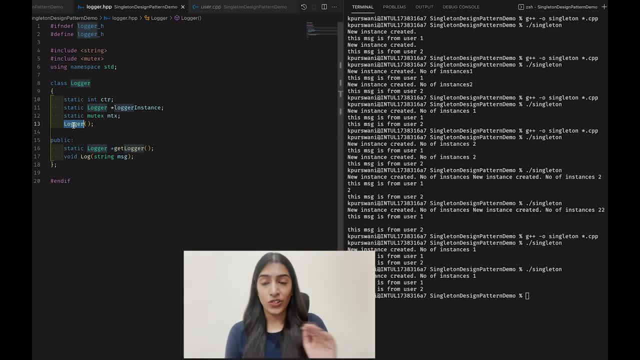 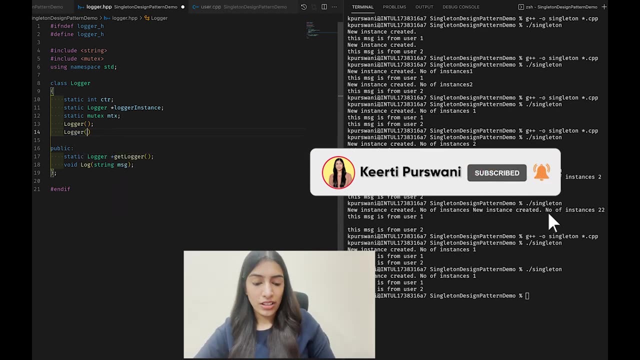 our users from calling logger constructor at all. so first we have to make the copy constructor also private. second, we have to make the equal to operator overloading also as private. so we add those two things over here. so the ideal way would be to write logger const and make the copy. constructor also private. make the operator private and make the copy constructor also private and make the operator overloading also private and make the copy constructor also private and make the copy constructor also private and make the operator overloading also impossible by making it private. so operator equal to and make it as. 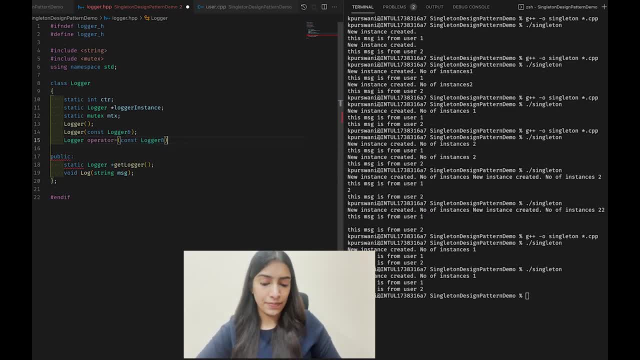 const logo and that's it. another thing, guys, for c plus plus people, only for people who code in c plus plus from c plus plus 11. making these functions private is not the only way to restrict users from calling them. there's also something called equal to delete. you can. 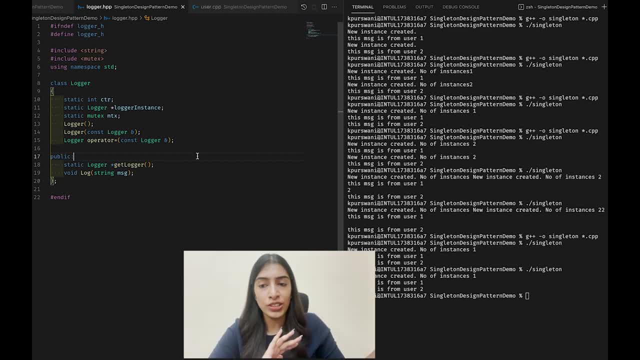 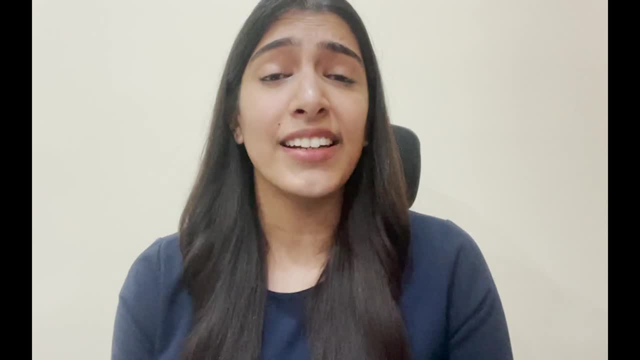 continue to put them in public section, but you just write equal to delete, so then users won't be able to call it. and that's it about singleton pattern. guys, this is a very common design pattern that you should know for sure. i hope i made things clear, simple and easy.